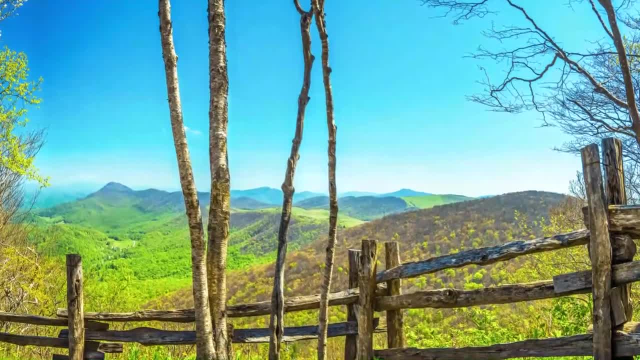 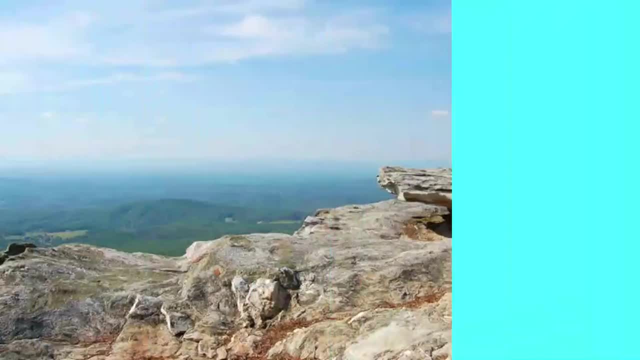 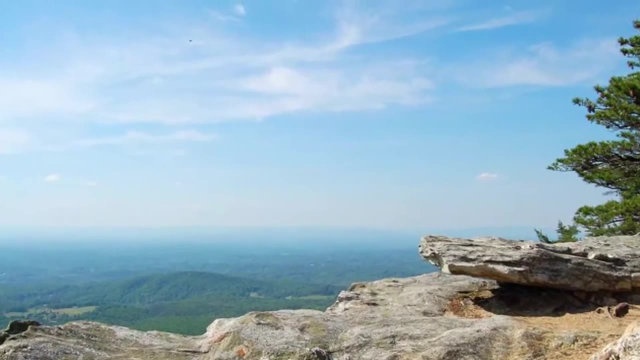 popular place for snowshoeing or even cross-country skiing. visit during the summer and you can look forward to some of the most picturesque hikes in north carolina. number four hanging rock state park, with five waterfalls, a mountain, a lake and a breathtaking rock outcroppings at 2 580 feet to. 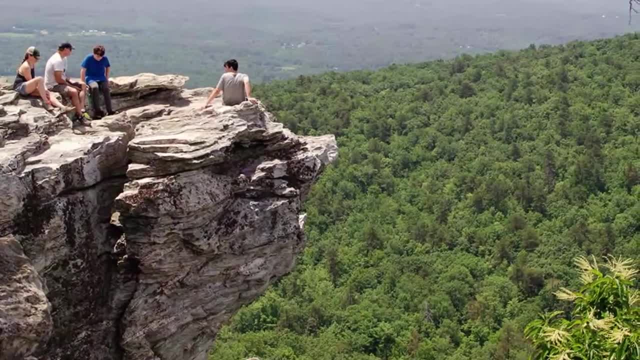 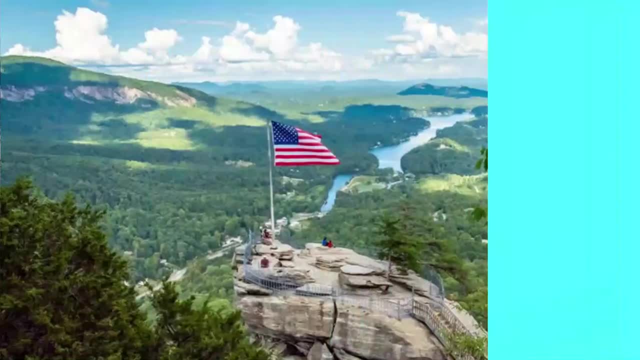 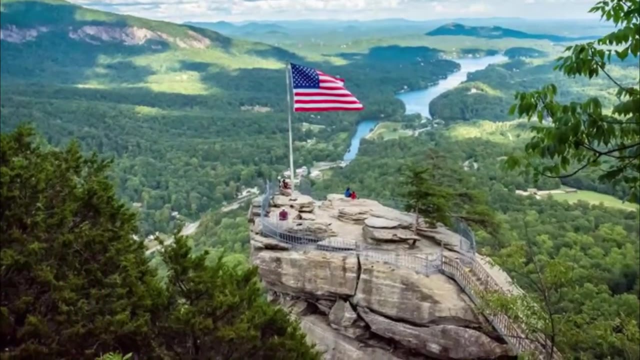 boot hanging rock state park is sure to fill up a whole day visit during the summer and you can look forward to some of the most picturesque hikes in north carolina. number five: chimney rock state park. chimney rock is seriously spectacular, given that the state park spans 5 700 acres. where does one? 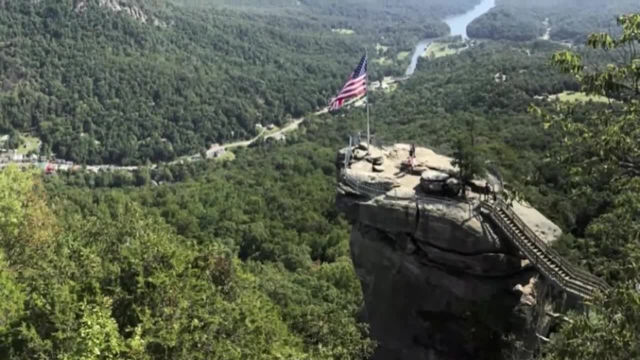 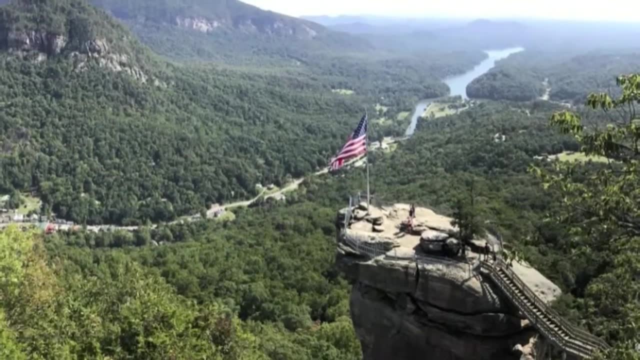 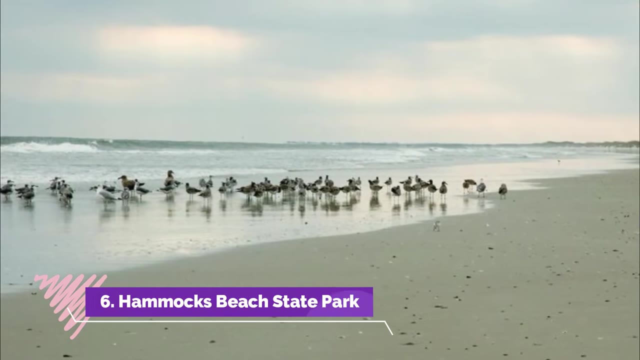 even begin between the 404 feet waterfall hiking, rock climbing and the legendary boulder with an elevator ride to the top. chimney rock belongs at the top of every outdoor enthusiast's bucket list. number six: hammocks beach state park, spanning from the mainland to the islands the park offers. 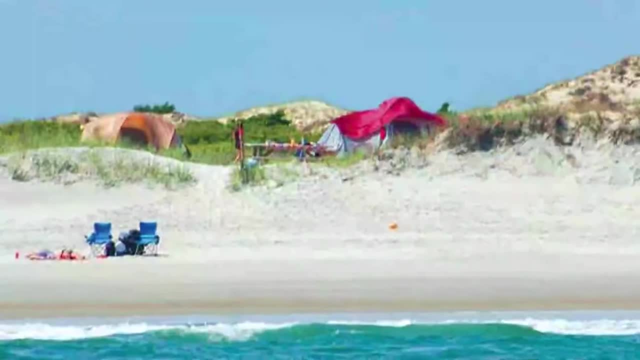 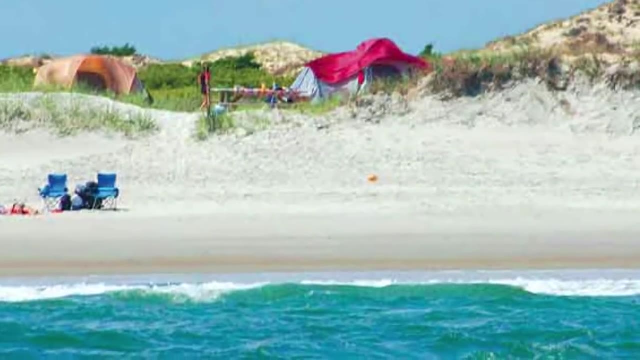 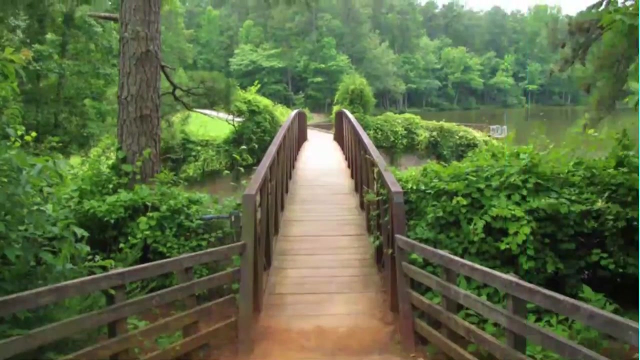 to the beach, maritime forest, salt marshes and tidal creeks. and camping on the beach, yes, please. there's nothing more peaceful than waking up to the sound of ocean waves and having the whole day to feel the sand between your toes. number seven: william b. william b- umstead state park. near raleigh awaits 5 000 acres of gorgeous scenery just asking to be explored. experience trails, lakes, canoeing and scenic overlooks. when you venture to this beloved and peaceful state park in north carolina, number eight pilot mountain state park, right outside of the piedmont, is one of the last remaining remnants of the swear town mountain chain. you can go rock. 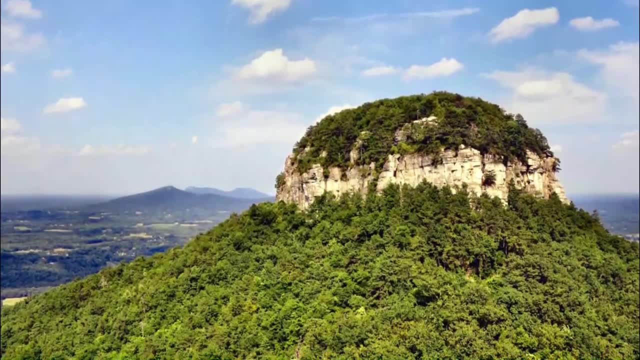 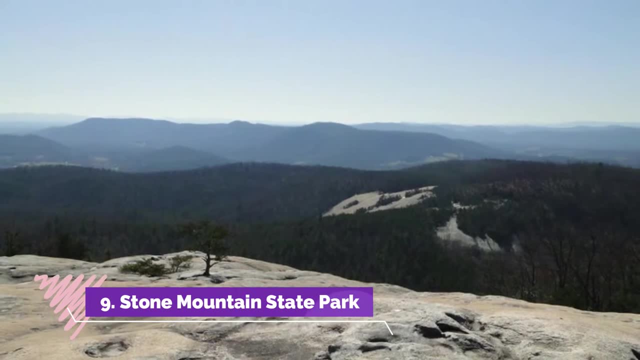 climbing, hiking or just take in all the glorious views at the top of this iconic north carolina landmark. number nine. stone mountain state park is one of the most famous and most popular state park mountain state park. rising 600 feet above the peacefully valley floor, stone mountain is one. 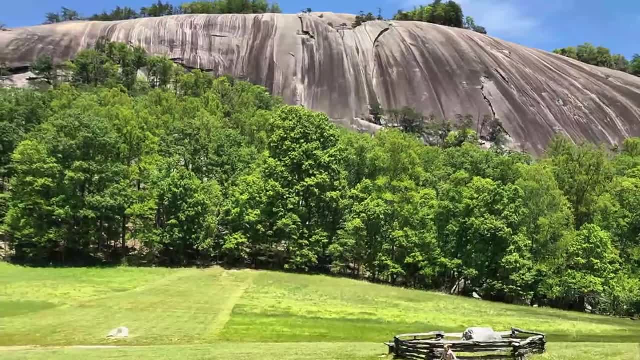 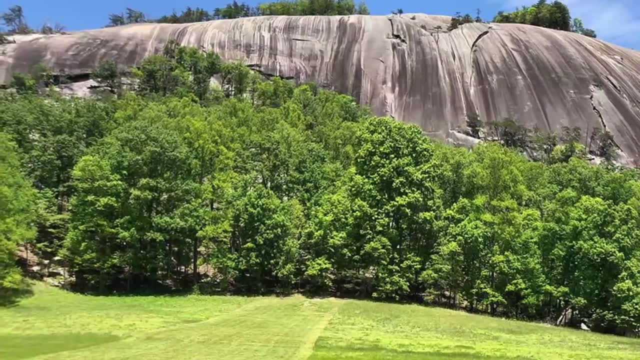 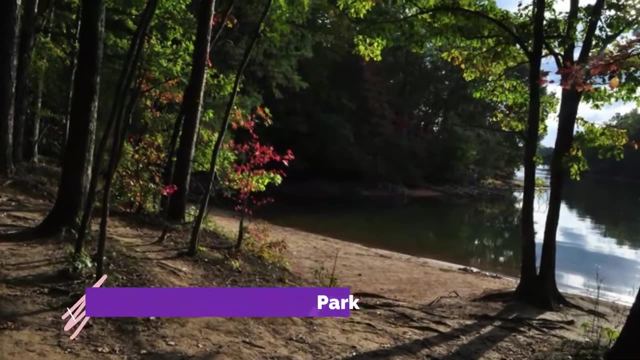 of north carolina's most unique attractions. dip your toes in the river, cool off by the waterfall, visit the 19th century homestead and enjoy the blue ridge mountain views. number 10: lake norman state park. at lake norman state park, you'll enjoy exquisite lakeside views and extensive hiking.